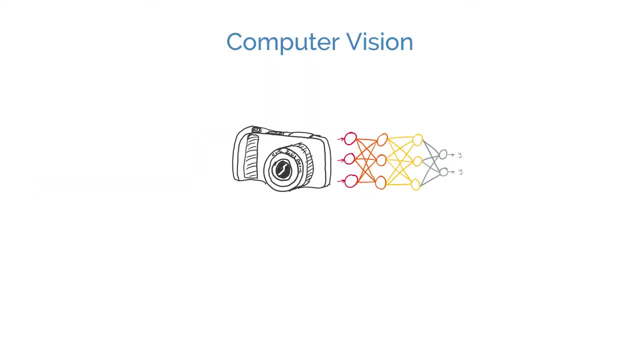 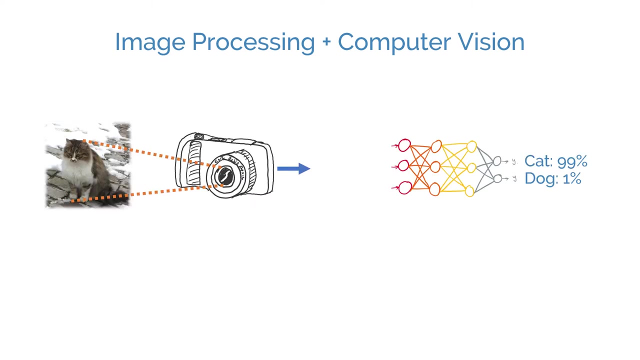 Computer vision, on the other hand, focuses on making sense of what a machine sees. A computer vision system inputs an image and outputs task-specific knowledge such as object labels and coordinates. Computer vision and image processing work together in many cases. Many computer vision systems rely on image processing algorithms. 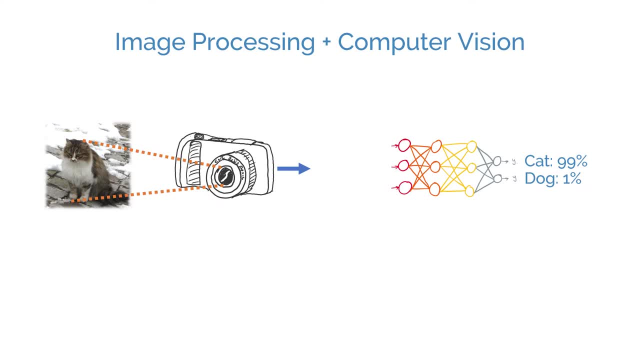 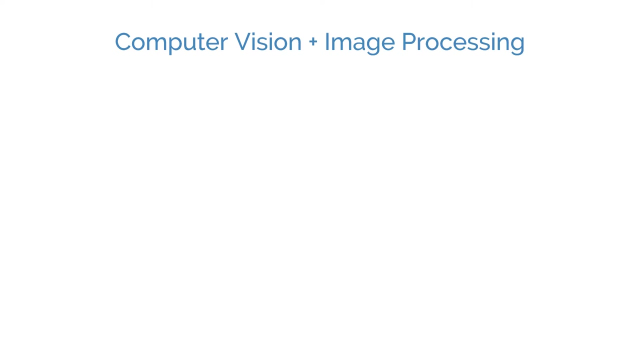 For example, computer vision systems rarely use raw imaging data that comes directly from a sensor. Instead, they use images that are processed by an image signal processor. The opposite is also possible. It wasn't common for an image processing algorithm to rely on computer vision systems in the past, but more and more advanced image processing methods. 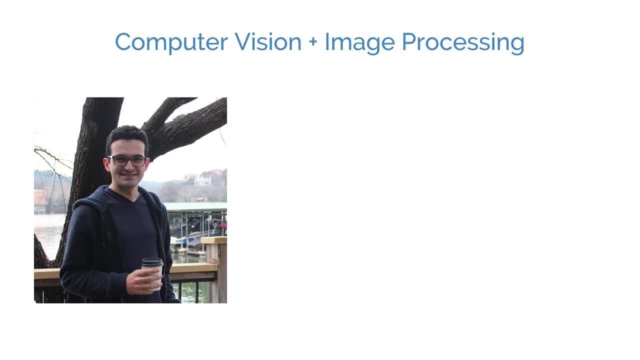 have started to use computer vision to enhance images. Face beautification filters, for example, use computer vision techniques to detect faces and apply smoothing filters, such as bilateral filters, selectively. They can do more advanced stuff, such as enhancing eye clarity or emulating a spotlight by detecting facial landmarks and tuning the images locally. 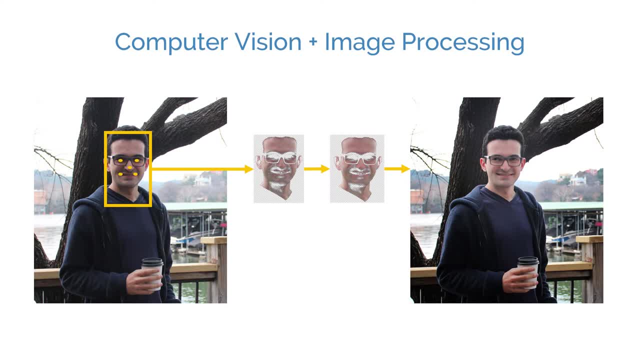 I know the result you see on the right doesn't really look good. It looks very artificial. I did it on purpose, though, to show the difference better. Another key characteristic of computer vision is the use of machine learning. We have talked about machine learning in the earlier videos, but if you're not familiar with the concept, 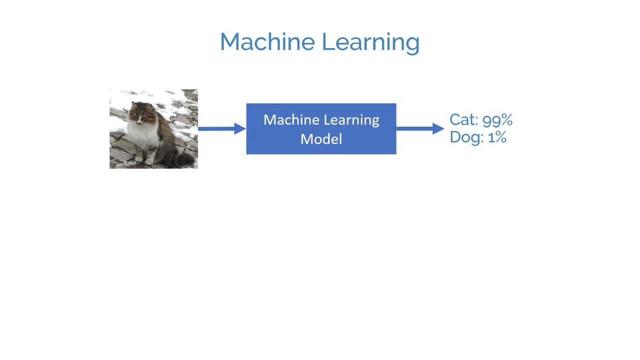 it's a field of study that focuses on teaching machines how to perform a certain task, given a set of examples. For example, we can build a model that can tell the difference between a cat and dog after being trained on pictures of cats and dogs. 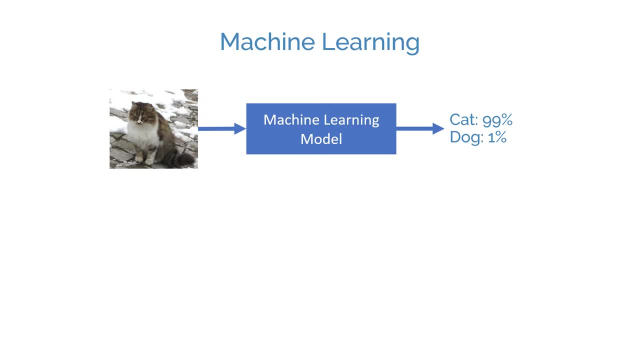 It's true that computer vision heavily relies on machine learning, but that's no longer a differentiator. Many advanced image processing methods also use machine learning models to transform images to accomplish a variety of tasks, such as applying artistic filters to an image tuning. 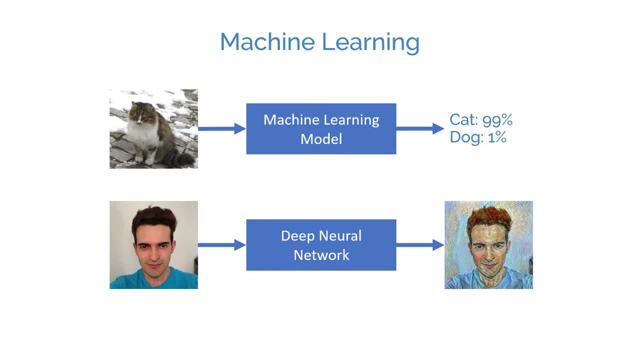 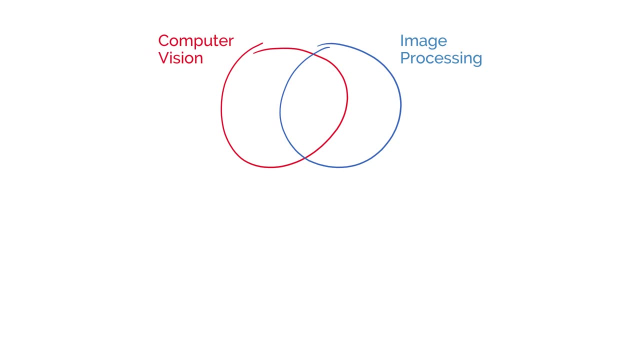 an image for optimal perceptual image quality or enhancing details to maximize the performance for computer vision tasks. It's worth mentioning that there isn't really a hard line between these two fields. The line between computer vision and image processing gets blurry when you do pixel-to-pixel.